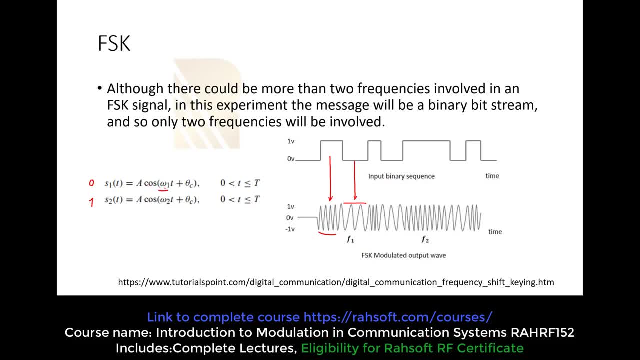 which is A cosine omega 1 T. The frequency is omega 1 and for a data one, if we have a data one or level high, let's say: well, it doesn't mean that we always have one volt, but we can assume that it's a high level. We are going to send the A cosine omega 2 here. This is a different frequency. 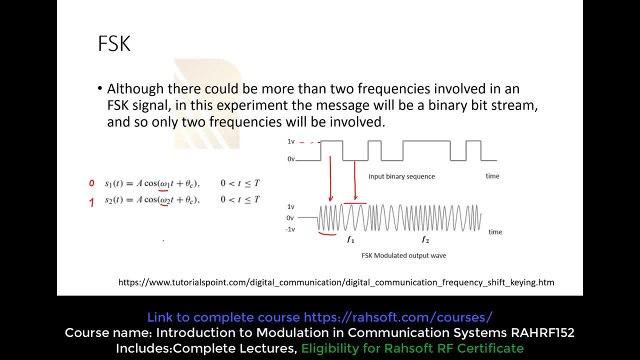 So in this experiment the message will be a binary bit stream and only two frequencies will be involved, because we have two levels here. But again, we can change this and we can have different kind of levels. For example, we can have four levels, four frequency levels. It means that 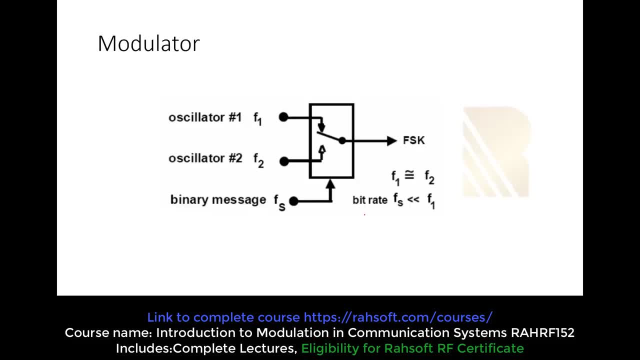 we are going to need more bandwidths. So, without wasting time, let's start a modulator. So here we can see the concept of FSK modulation. It's very simple actually. We have two oscillators. So the first oscillator is producing F1.. So we can say that this 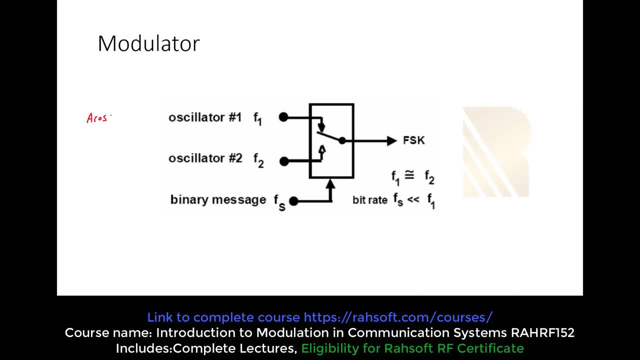 oscillator is producing A cosine. let's say, omega 1 is the angle frequency, So omega 1 T plus. we are going to have the initial phase. It doesn't matter on here, This is going to be A cosine: omega 2 T plus phi zero. This is the initial phase as well. So what are we doing here is very simple: It's a switch and the 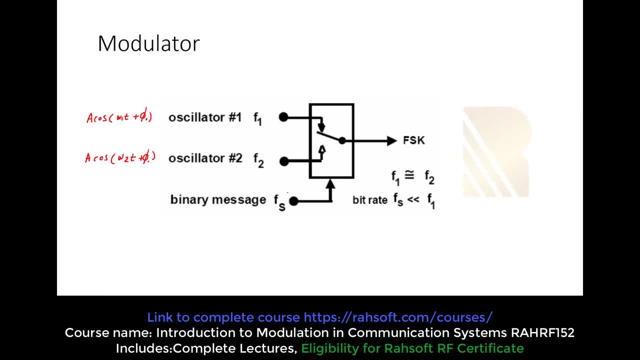 binary data. when the binary message is, for example, one, we are going to switch one of this. for example, when this is zero, let's say, we are going to switch the oscillator one. So at the output we are going to have omega 1 frequency. and when we have a data binary and the data one is when it's high, we're 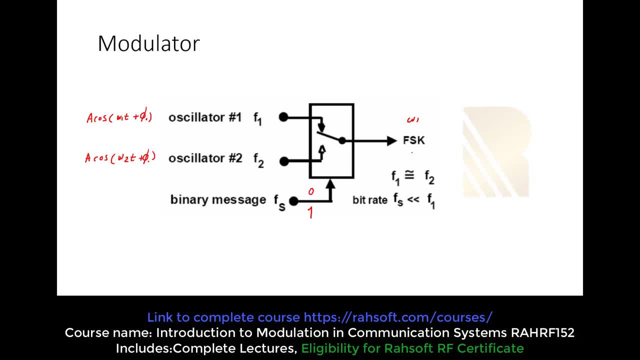 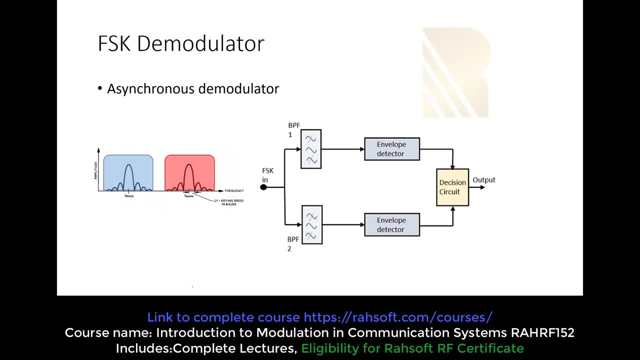 going to switch the below one here, F2, and we're going to have omega 2 at the output. So this is how the FSK modulator works. What about the demodulation? We are going to explain this FSK demodulator. So first of all we have to talk about the output spectrum of the FSK. 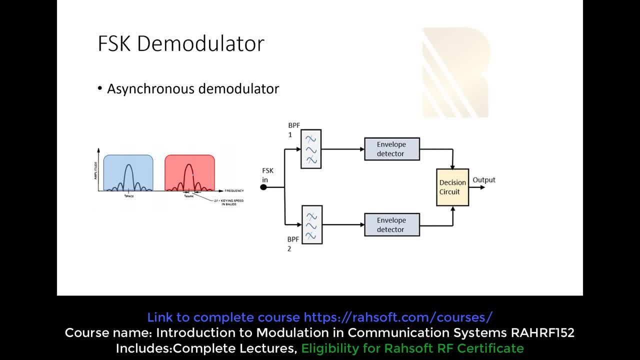 demodulator. So we are going to have this kind of output, this kind of frequency spectrum because, as we talked before, we are going to send two waves. We said A cosine omega 1 and A cosine omega 2.. That's why we are going to have two bands So we can say this: this is FSK output: modulated signals.